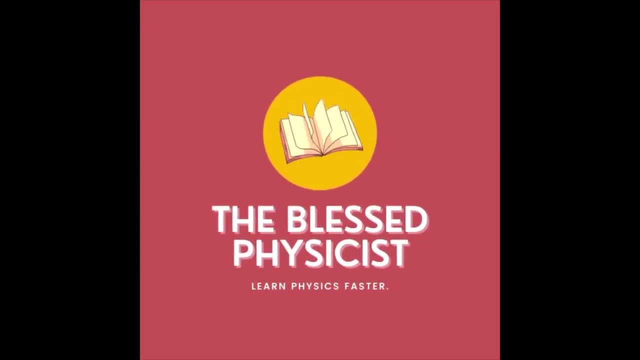 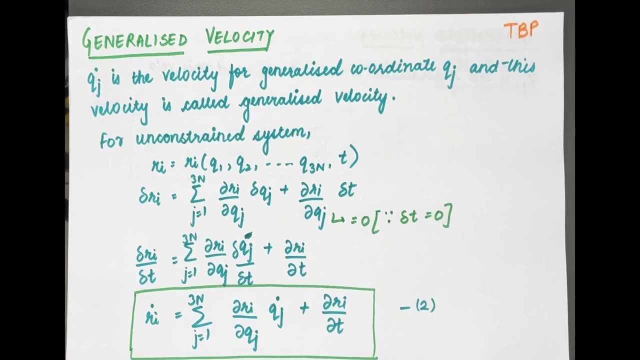 Hello and welcome back to my channel, The Blessed Physicist. In the previous video we talked about generalized displacement and in this video we are going to talk about generalized velocity. When we take time derivative of the generalized coordinate qj, we represent it as qj, dot That. 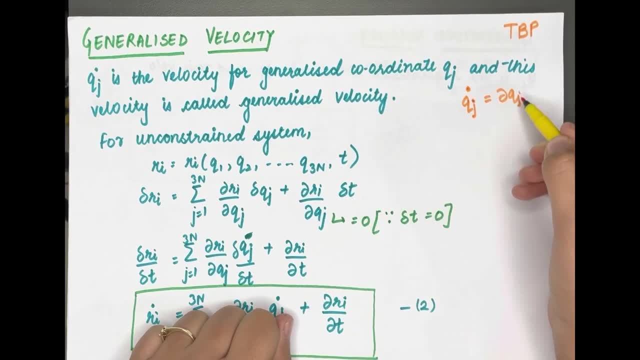 means qj dot is equal to curly qj by curly t. Okay, so qj dot is the velocity for generalized coordinate qj, and this velocity is called generalized velocity For unconstrained system. why unconstrained system? because we know that the system is free to move in all the possible. 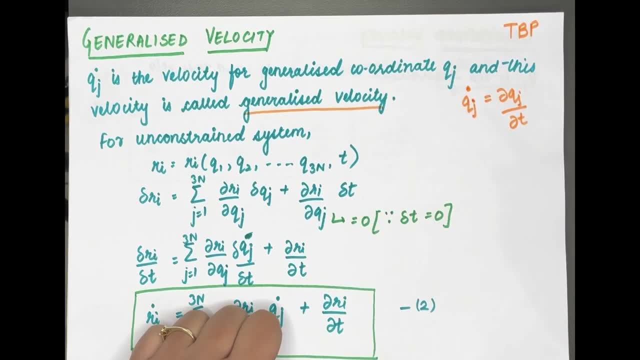 direction for unconstrained system and the possible number of directions for unconstrained system Is 3n. We have studied this in the previous videos. Okay, so for unconstrained system, ri is equal to ri, q1, q2 up to q3n and t. So it depends on the coordinates q1, q2 up to q3n. 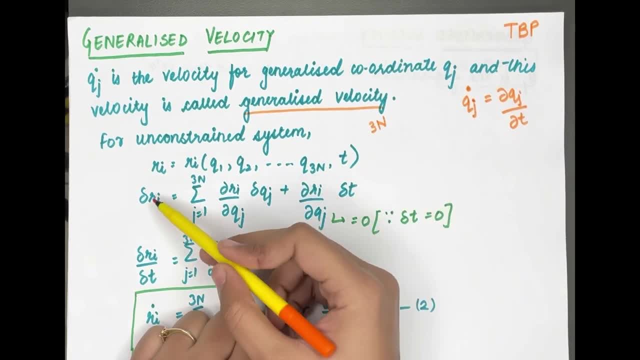 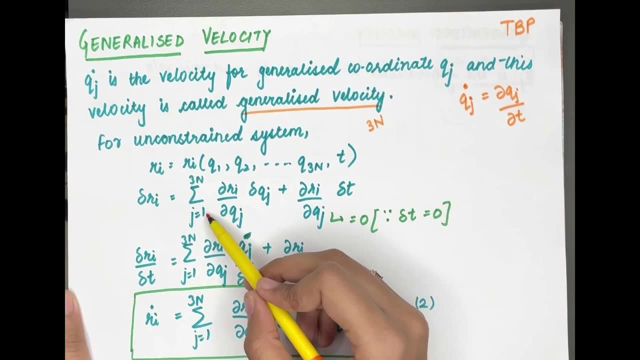 and time t How we take del ri. in the previous video we have already studied about all this. Del ri is equal to summation j, So del ri by summation j is equal to one to three and curly ri by curly qj, del qj plus. 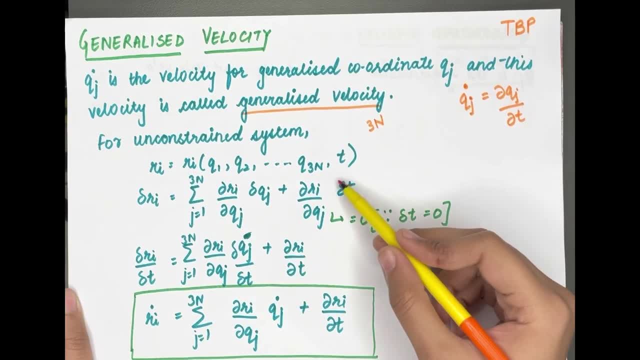 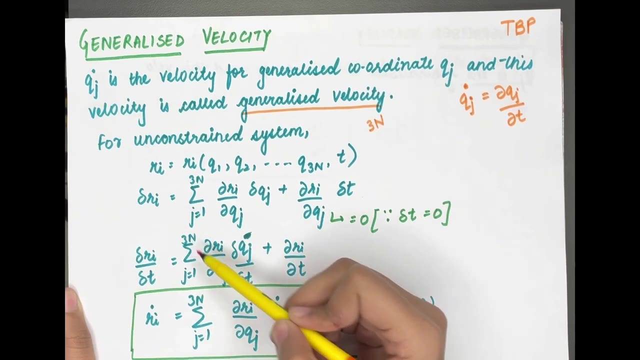 curly ri by curly qj del t. And in the previous video only I have told you that del t is equal to 0 because we have kept time t fixed. So the time derivative of del ri is del ri by del t is equal to summation j is equal. 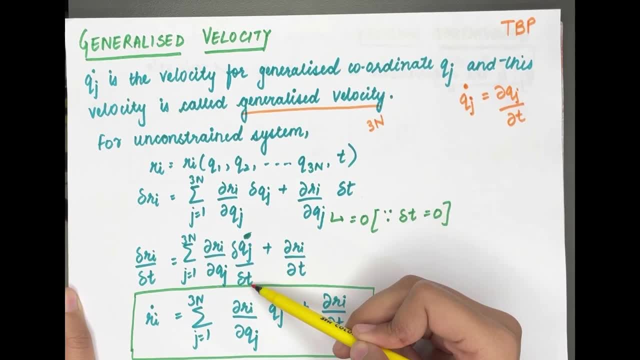 to 1-3: n. Curly ri by curly qj, del qj, del qj. So we are going to take this in the current situation for unconstrained system and the time derivative is same with this: del ri by qj by del t plus curly ri by curly t. So we will represent the time derivative as ri. 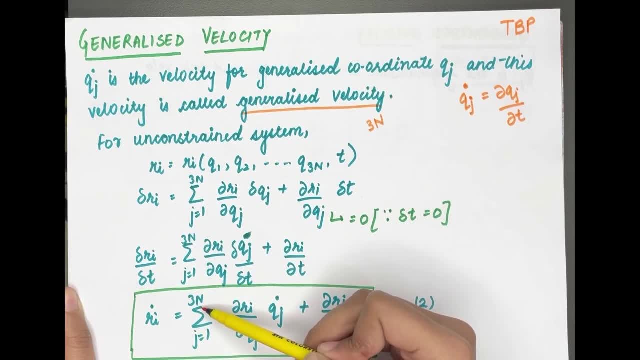 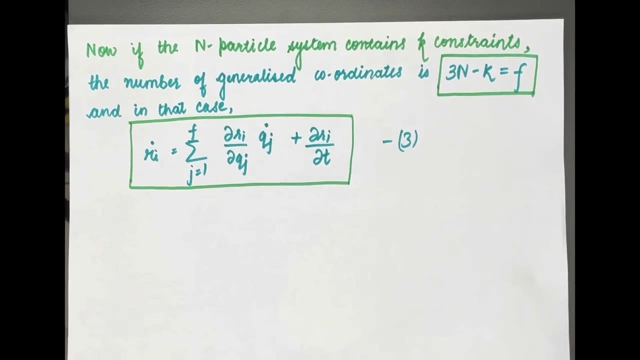 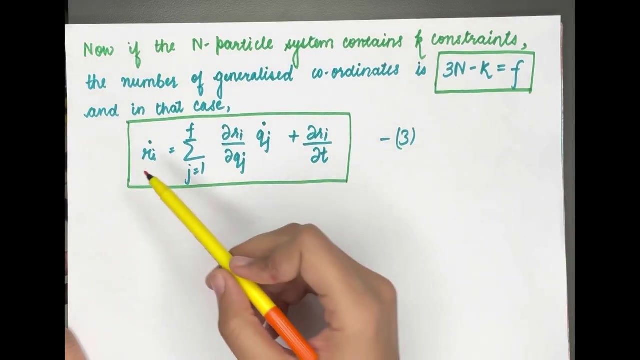 dot. ri dot is equal to summation, j is equal to 1 to 3. n. curly ri by curly qj, qj dot plus curly ri by curly t. Now, if the n particle system contains k constraints, the number of generalized coordinates is 3. n minus k is equal to f, and in that case ri dot is.